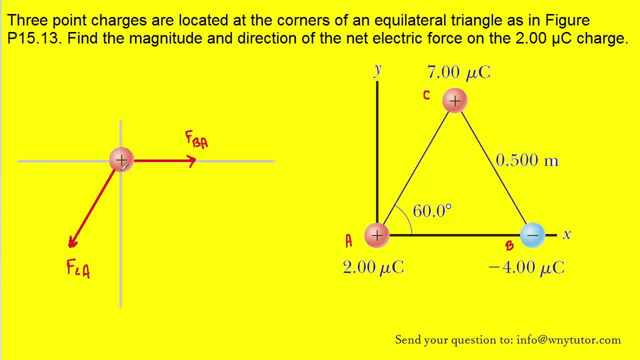 Now it turns out that there are two electric forces acting on the positive charge. but before we can understand those two forces, please take note that we've labeled the charges arbitrarily with the letters A, B and C, A being the charge whose force we are trying to determine. 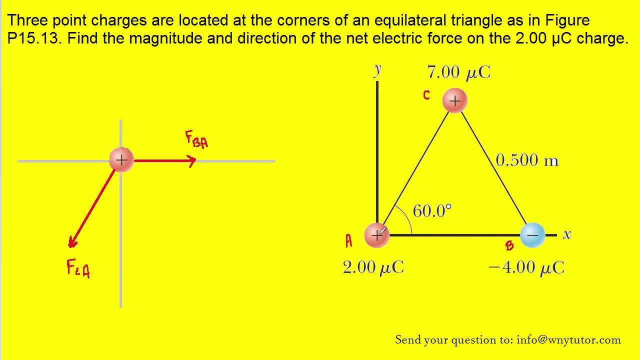 Now charge B, being negative, is going to attract charge A and that means it's going to pull it to the right and along the positive x-axis. So we have drawn a force acting along the positive x-axis and we have labeled it as FBA. 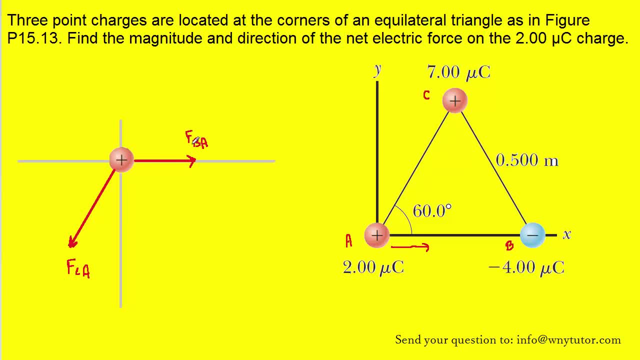 That simply means the force that charge B is exerting on A Charge C is positive and since charge A also is positive, there's going to be a repulsive force acting. So, in essence, charge C is going to be pushing charge A away from it. 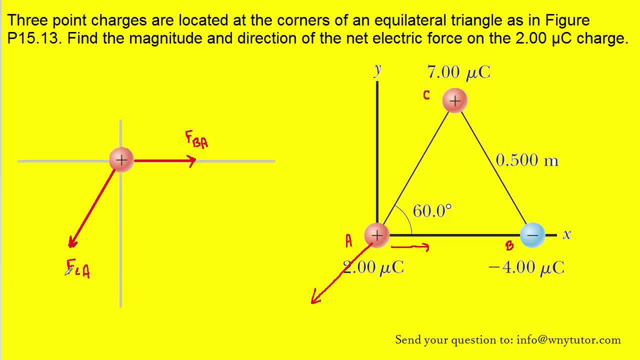 and we can label that force, as we have done in the free body diagram, as FCA. That is, the force that charge C is exerting on charge A, Again a repulsive force. Now it turns out that this angle right here is going to be 30 degrees, although we'd like to justify that. 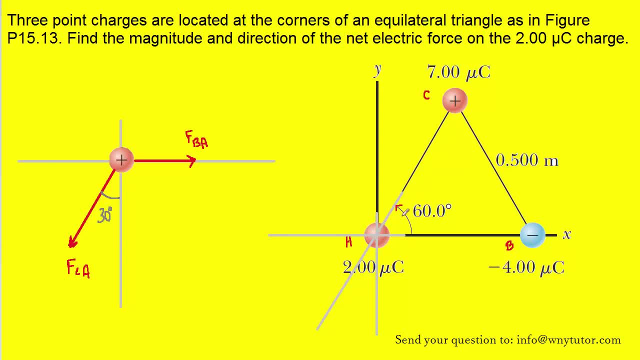 So we'll come back over to the original diagram. The question noted that this angle right here is 60 degrees, which makes sense because it's an equilateral triangle. Now we remember from high school geometry perhaps, that if this angle is marked 60 degrees, 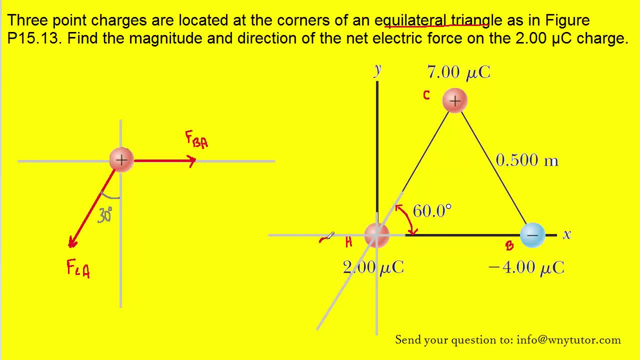 then the angle immediately across from it- it's known as a vertical angle- will also have a measure of 60 degrees. Now, of course, the angle between the x and the y-axis is 90 degrees, So from there to there would be 90 degrees, and that means that this angle right here will indeed be 30 degrees. 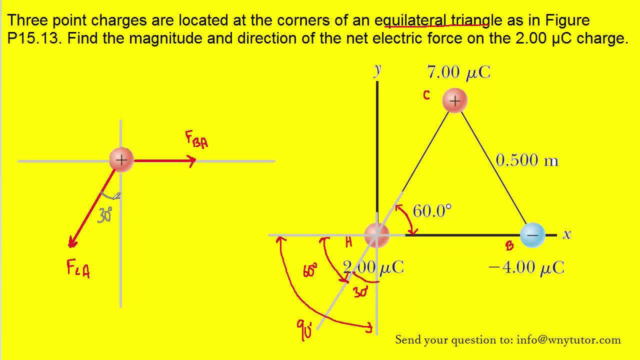 And so that's where we're coming up with the 30 degrees marked in our free body diagram. Our next step is to break these forces into their x and y components. Notice that the force marked FBA has only an x component. It's directed exactly along the x-axis, so there's no need to break it into any components. 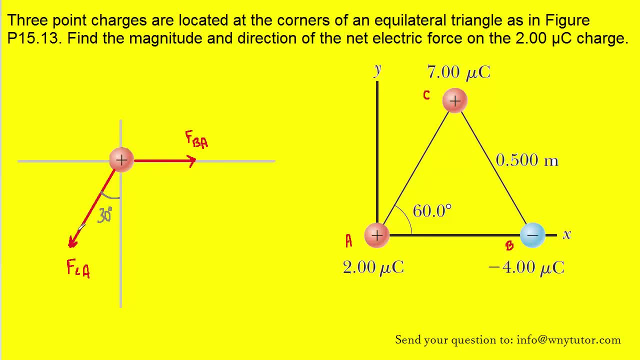 FCA, on the other hand, is acting at an angle, and so we will need to break it up into a y and an x component. Now we'll notice that the y component, which is pointing down, is adjacent to the 30-degree angle. 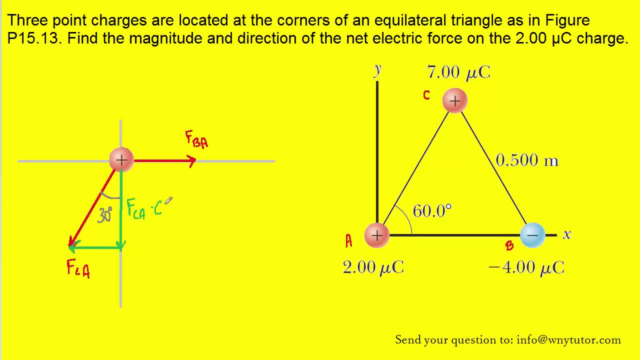 So we can label that component as FCA times the cosine of 30 degrees. and then the x component, which is pointing to the left, is opposite to the 30-degree angle, So that can be labeled as FCA times the sine of 30 degrees. 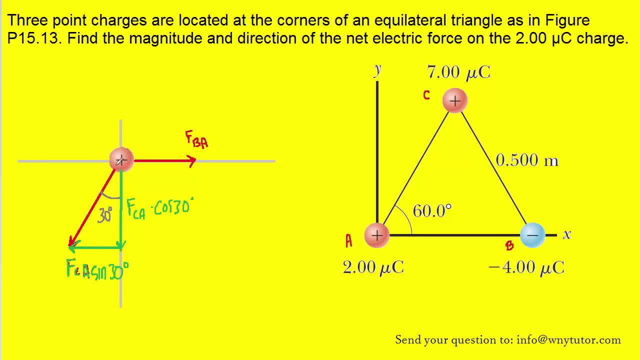 Now, once we've broken the forces into the y and x components, we can get rid of the red resultant force, because we really only need to be working with the components in the later calculations. So let's remove this red resultant force, FCA. 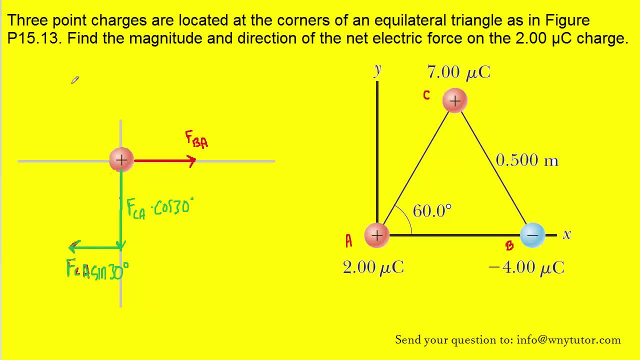 Now we don't want to forget that FBA and FCA are both electrical forces and they will obey Coulomb's law. Let's take a look at that equation. We have a Coulomb's constant multiplied by the magnitude of the two charges divided by the distance between the charges squared. 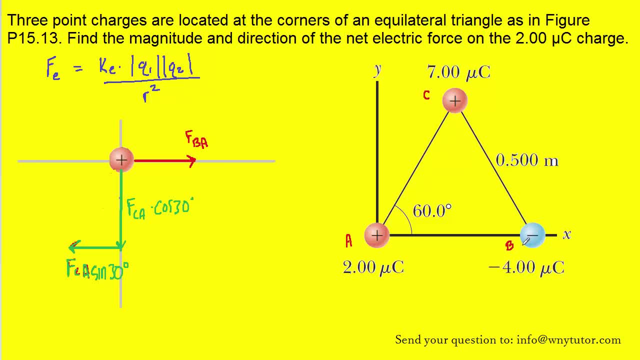 So, for example, if we look at FBA, we can see that we have the charge labeled negative 4 µC and positive 2 µC, with a distance between them of 0.5 m. So we can actually replace FBA with an expression that is equivalent to the Coulomb's law of force. 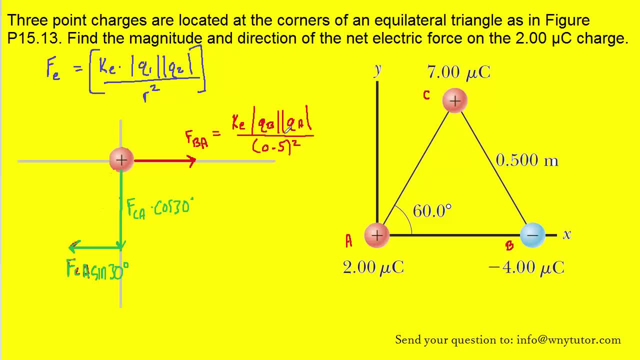 For now for the charges. before we plug in the numbers, we'll just use QB and QA to represent the charge of object B and object A, A. We can do the same thing with FCA. We'll now notice that the sum of the forces in the x. 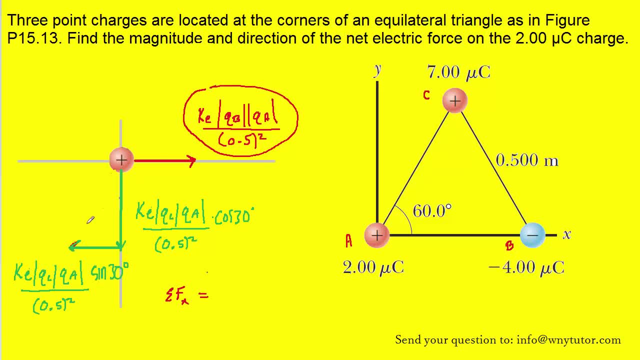 direction will be this positive component right here, added to this negative component right here. Those are the two component forces that are acting in the x direction. So let's fill that into the sum of the forces in the x direction. Now, perhaps that's a bit of a messy expression, Keep in mind. 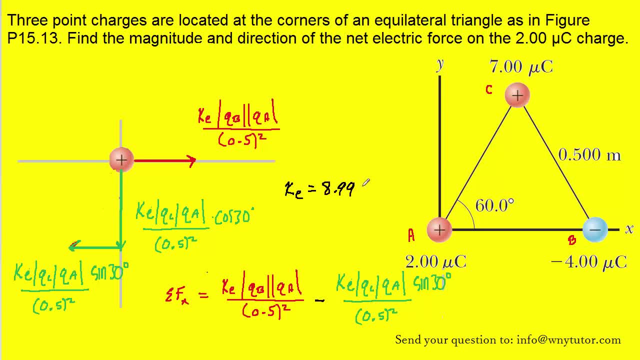 please that KE. the Coulomb's constant is equal to 8.99 times 10 to the ninth. So that's what you're going to plug in right there and there. QB would represent the charge on sphere B, which is labeled as negative 4 microcoulombs. but that needs to be converted into the standard unit of. 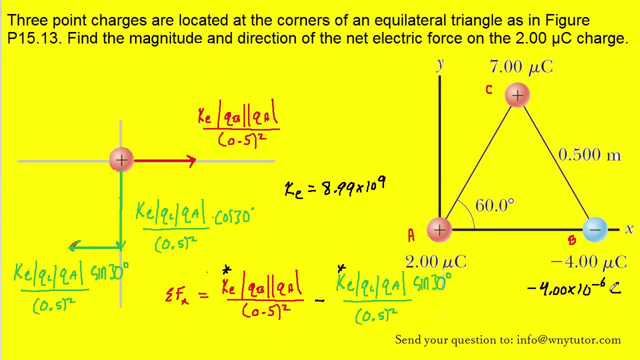 Coulombs. So when you plug that in it should be negative 4 times 10 to the minus 6th Coulombs. Same thing with QA. They gave that as 2 microcoulombs but you're going to have to plug in 2. 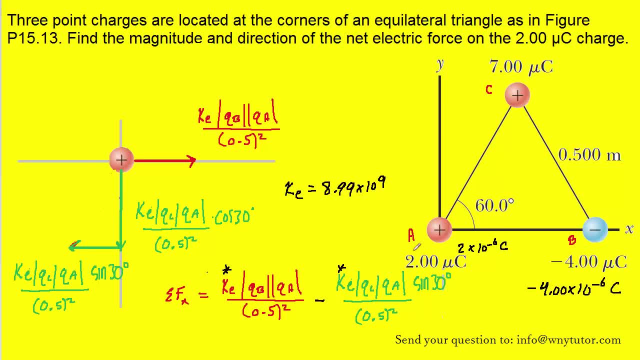 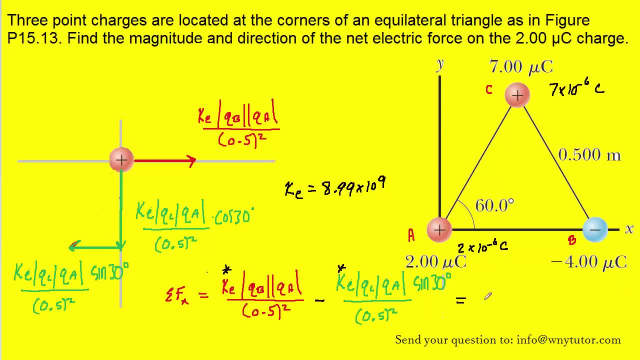 Coulombs, We can plug in all of this into our calculator and you should get approximately 3.6 times 10 to the minus 2, and the unit will come out in Newton, since everything else was in a standard unit. So that's the sum of the forces in the x direction. Notice that the sum of the forces 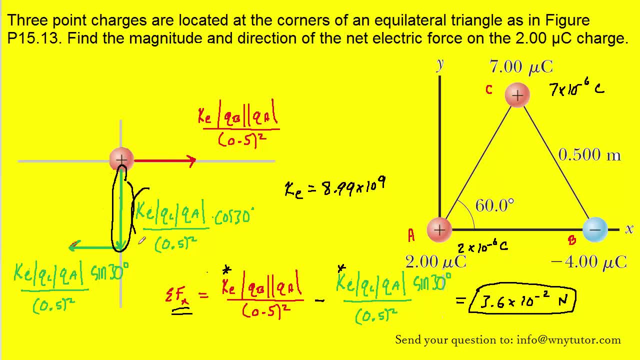 in the y direction will simply be this single downward component that's pointing down along the y axis. So this is the sum of the forces in the y direction. We just have to make sure we assign a negative to it, since it's pointing downward. So in other words, the sum of the forces in the y 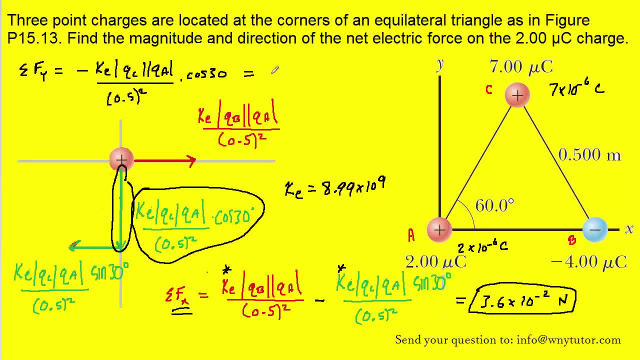 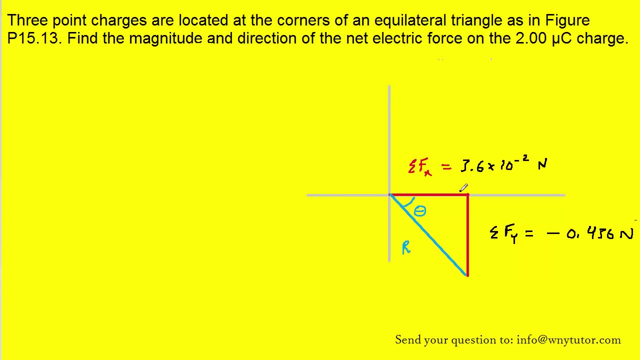 direction is equal to this quantity. here, If we plug this all into our calculator, we get approximately negative 0.436 Newtons. So now that we have the sum of the forces for the y direction and the sum of the forces for the x direction, we can find the resultant. The net x force is positive. 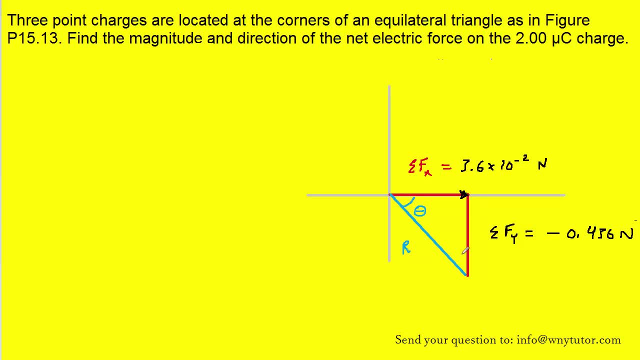 so it's pointing to the right along the positive x axis. The net y force is negative, so we've projected it downward. The resultant would be a line drawn from the origin to the tip of the y force, And that forms a right triangle. We can apply the Pythagorean theorem. You can plug in the known values for net fx and net fy. 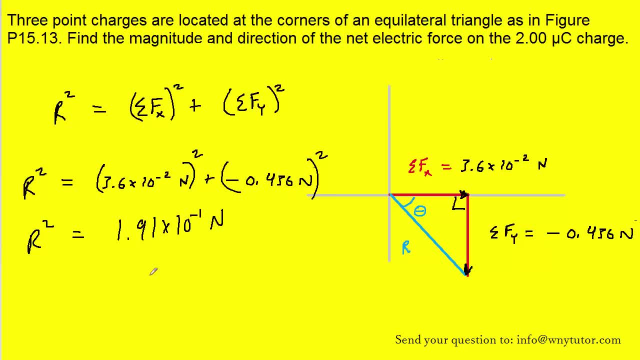 You get r squared is equal to 1.91 times 10 to the minus 1 Newtons squared, And then take the square root and you get approximately 0.438 Newtons for the magnitude of the resultant force. To find theta: 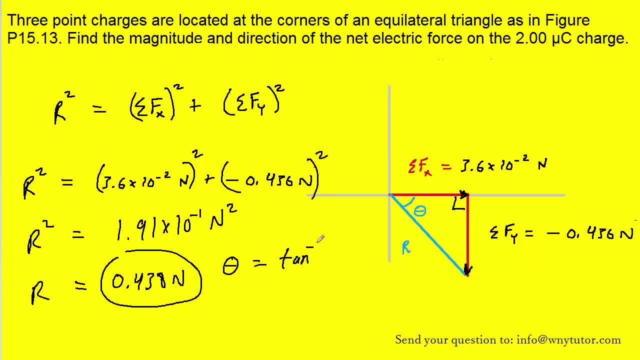 which is dipping below the positive x axis. you just have to take the inverse tangent of your opposite side, which was negative 0.436, divided by your adjacent side, which is the 3.6 times 10 to the minus 2. And you get approximately negative 85.2 degrees. Another way: 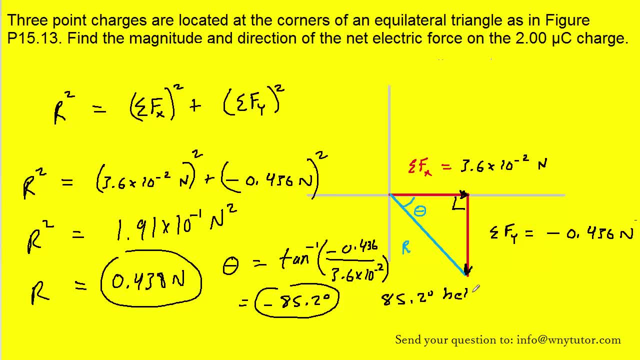 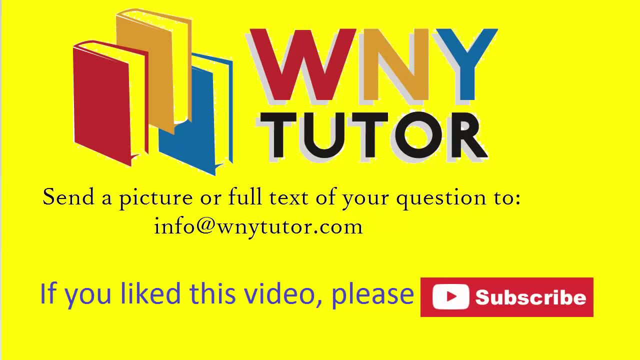 of representing. that would just be to say 85.2 degrees below the positive x axis. Thanks for watching this video. If you liked it, please subscribe to the channel so that you can stay tuned for additional videos. You're always welcome to send in your own question to the email address listed on the.